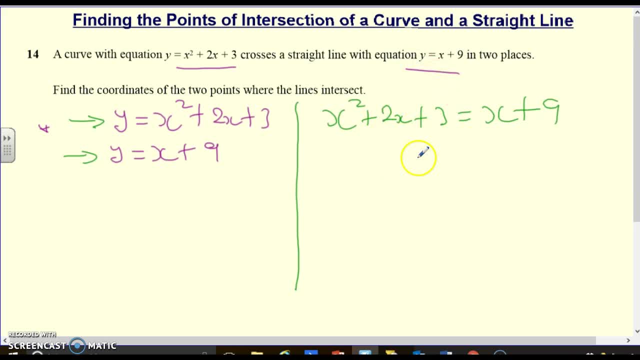 we want to find the point of intercession of a curve and a straight line. We want to be able to isolate the terms of this equation so that we end up with a quadratic equation of the form ax squared. add bx, add c equals to zero, so that we can work out what x is. 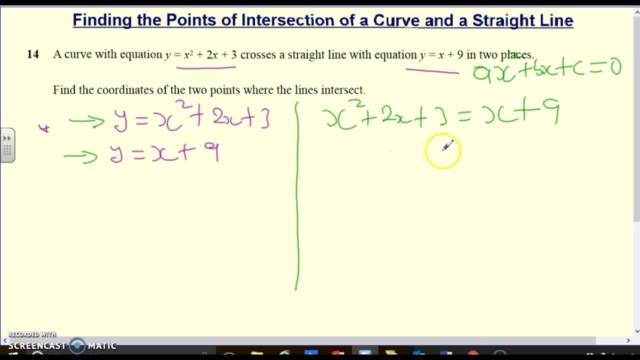 To do that, we would want to isolate our points. Let's now isolate our whole numbers. We'll do that by subtracting 9 from both sides, because we want to end up with a zero on the right-hand side. What else would we do? 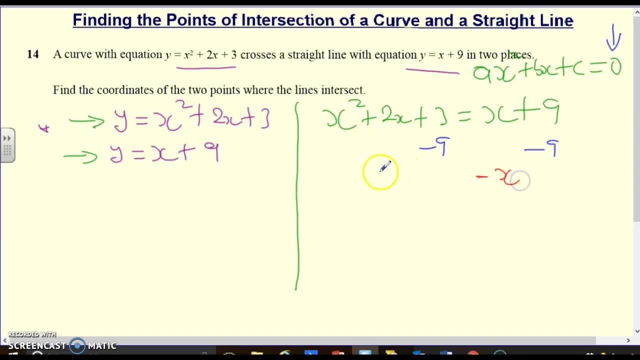 We will then eliminate the x as well from the right-hand side, and we want to make sure that we do it to both sides. We need to do it to both sides because of the power of the equal sign. Whatever we do to the left, we need to do it to the right. 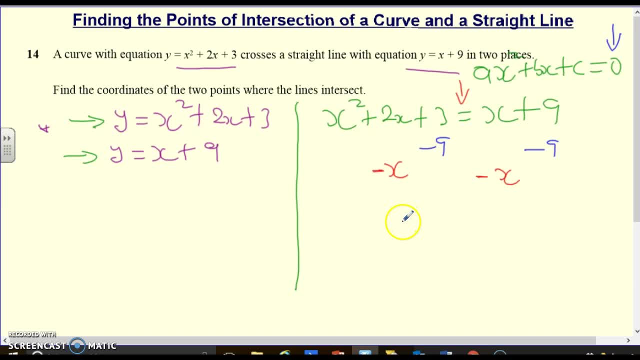 So that our equation remains balanced at all times. At this stage, then we can safely simplify both sides. x squared obviously would come down with no changes. And then we have 2x take away x. We have our positive 3 take away. 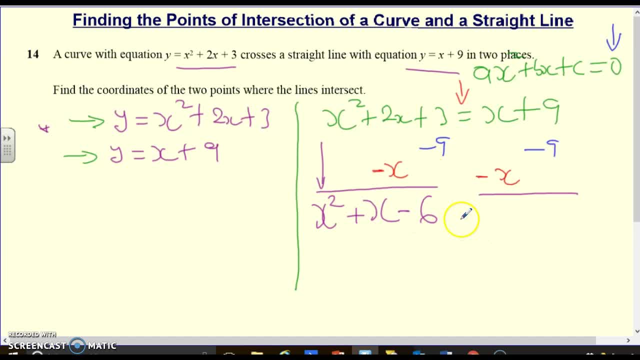 9, from both sides 9, and this now would equal zero. So we want to think of, at this stage, two numbers whose product will give us negative 6,, but whose sum will give us the coefficient of this x, which obviously is 1.. 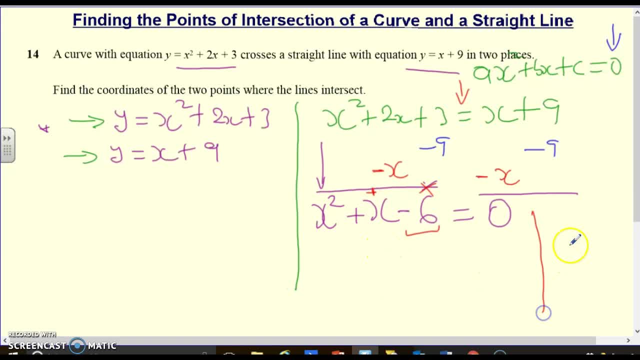 So what two numbers can you think of Now? we can then go through any two numbers, for example, that multiply to give us 6. So we have 1, 6,, 2, 3, and so on, And then ask ourselves: which of these two do we choose? 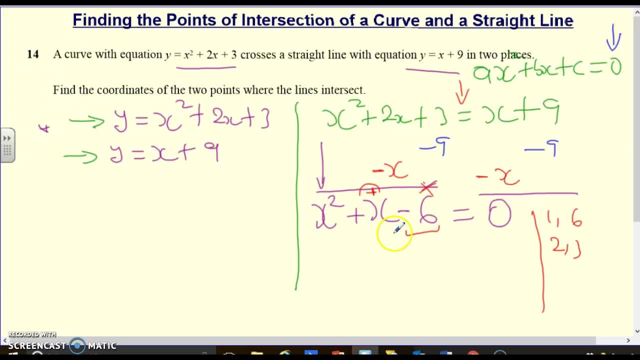 So that when we add both at some point, we will be ending up with a 1.. So that makes 2 and 3 our safest option. And in considering the 2 and 3,, which of these two numbers can I negate? 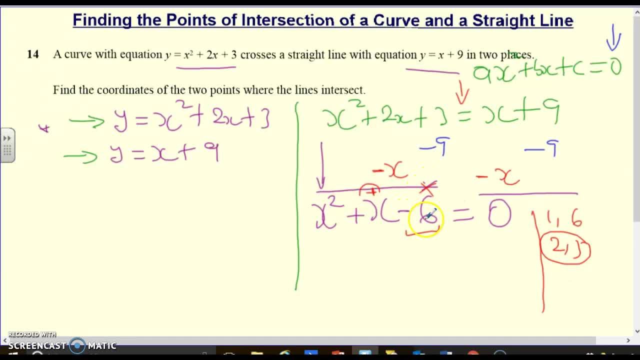 So that when I multiply I would still get a negative 6,, but then I would add to get a positive 1.. And so the safest answer is to negate the 2. Then all you do introduce your double brackets, So your answer then becomes x minus 2, x plus 3.. 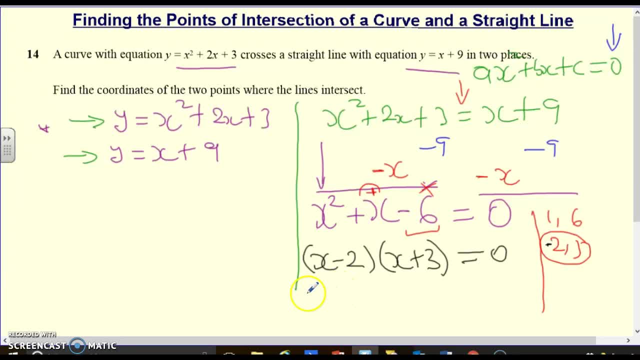 Okay, Right At this stage, this tells you that you have the product of two numbers and they give you zero. This would then mean that either x minus 2 is zero or x plus 3 is zero, Because one of them has to be zero for the product to be zero. 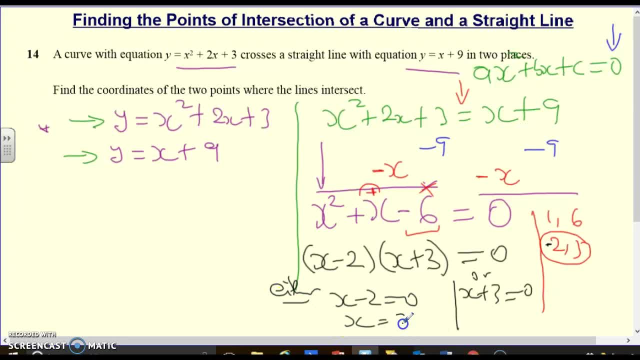 So this simplifies to x equals 2, or x equals negative 3.. Now, remember this: We're looking at the two points of intersessions In general. a quadratic curve of this form with positive coefficient of the x squared will have this shape, and a linear equation of this with a positive gradient will have this shape. 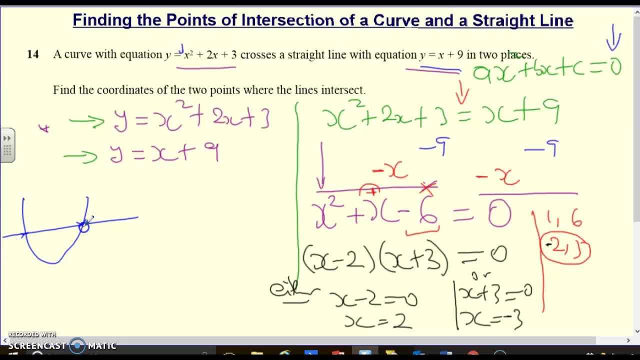 They will meet if we were using a graph at two points, And each of the two points will have a coordinate made up of x and y. Hence, having worked out what our x's are, we will need to substitute them into either of the four. 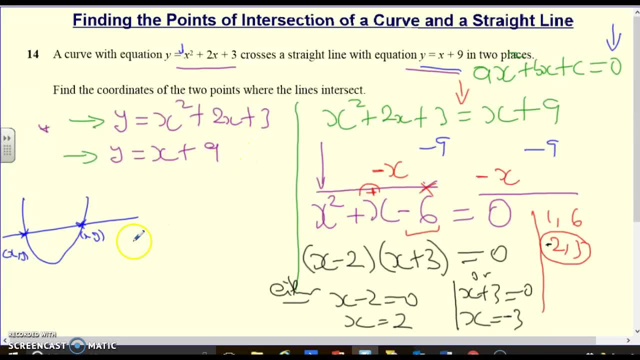 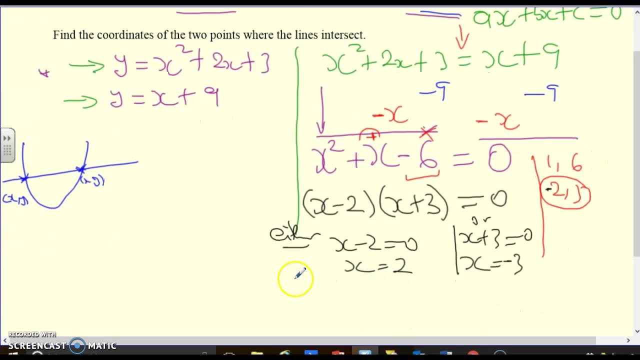 Okay, Okay, Of the first two of the equations to work out the corresponding y-value. So we say, if x is 2, then it would mean that y will be equal to 2 add 9.. That is using the second equation.